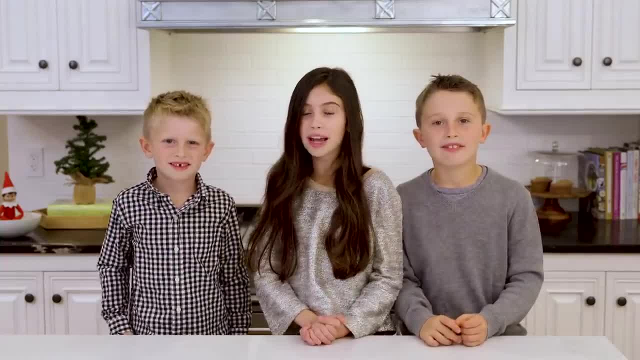 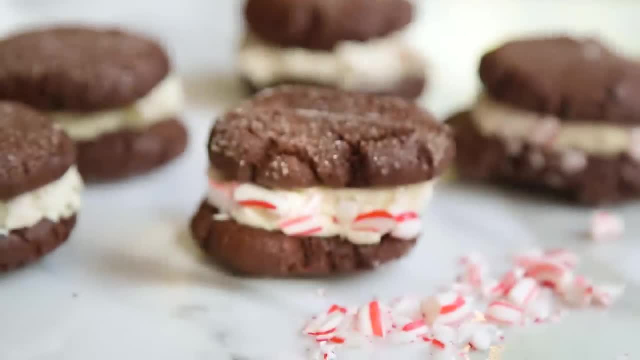 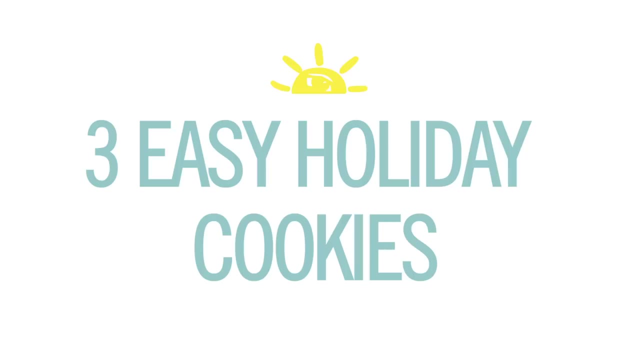 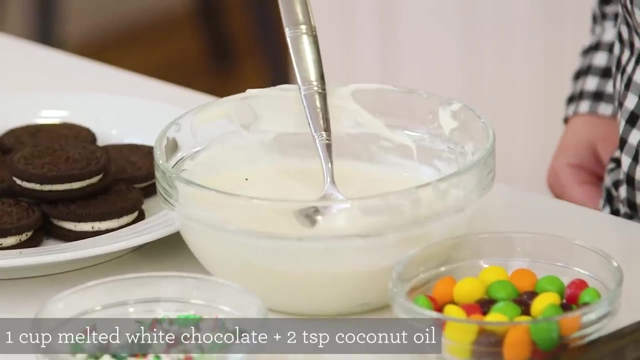 Hey guys, This year we decided to give our mom a break and we're making the Christmas cookies. Today we're going to show you three Christmas cookie recipes that kids can make themselves. They're easy but delicious- Yeah, they are. First, we're gonna make Oreo ornaments. My mom melted some white chocolate. She got some Oreos. 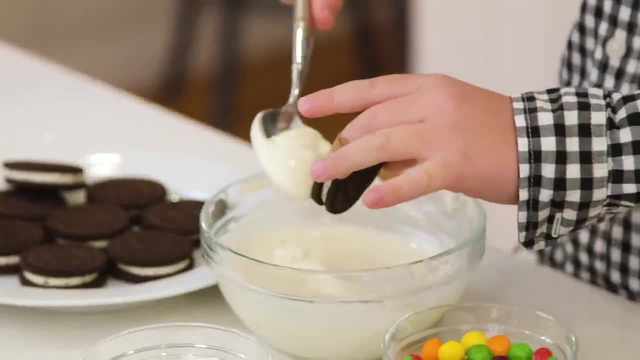 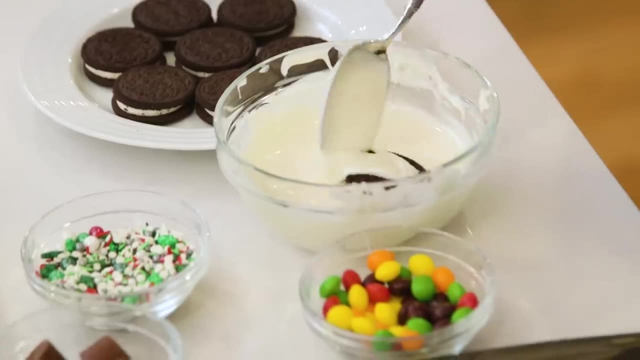 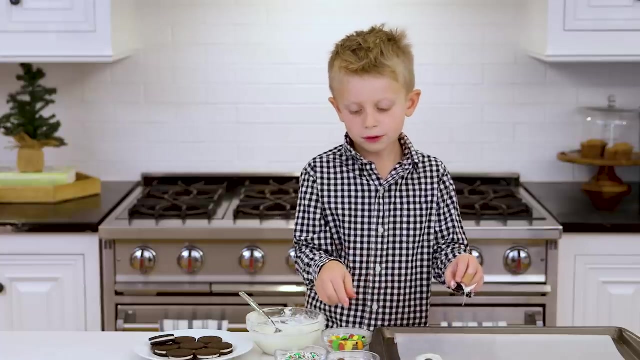 Now we're gonna pour some white chocolate on the Oreo. It's looking good. I think I'm gonna dip it. It might be easier. I'm just covering it and making it so it just looks like white chocolate. Now you're gonna put some. what are these called? Now we're gonna put a roll. That's the. 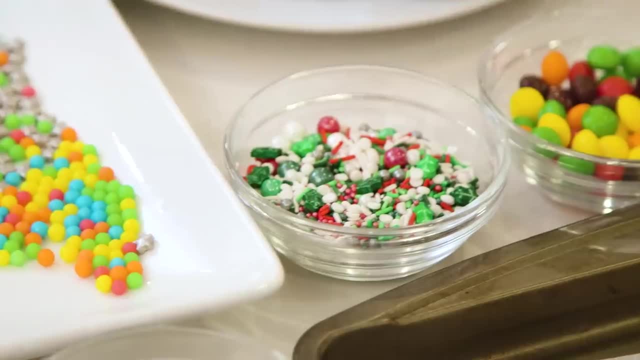 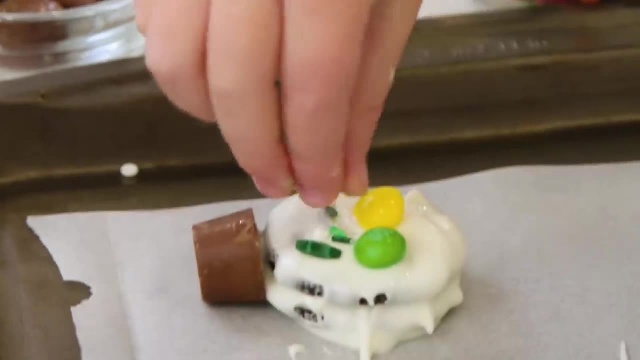 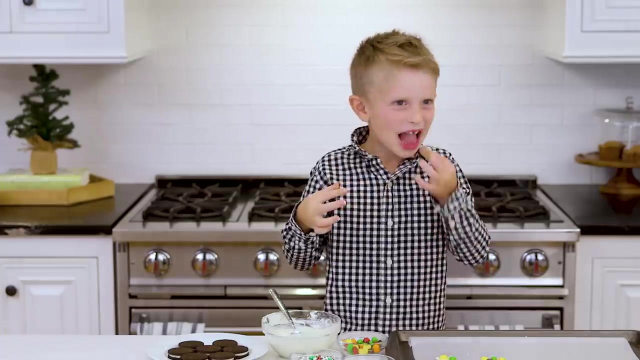 ornament hook. Now we're gonna decorate. I got some Skittles, I got some ornaments, I'm just gonna mix it up. I'm doing a pattern. You can do whatever you want. This is especially so much fun because I get to lick my fingers. Now you gotta wash them, Goose. 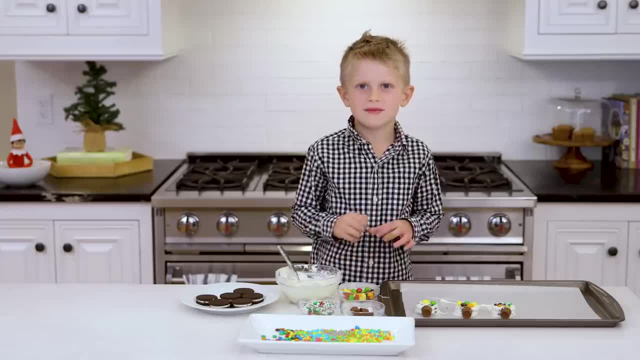 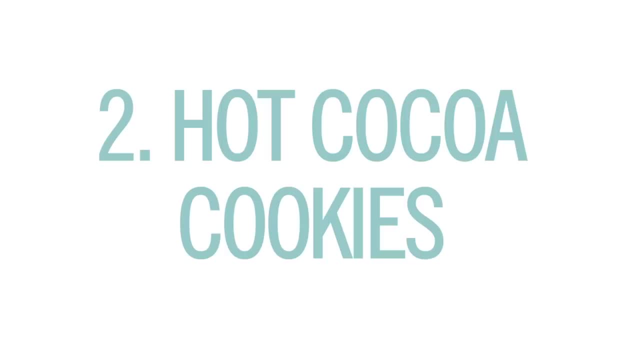 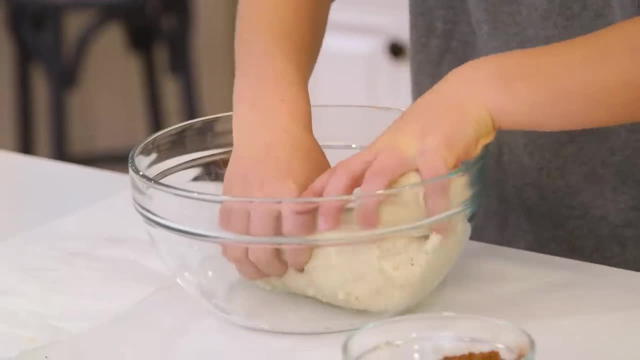 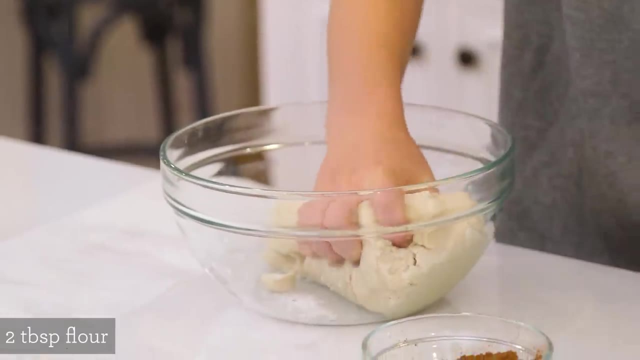 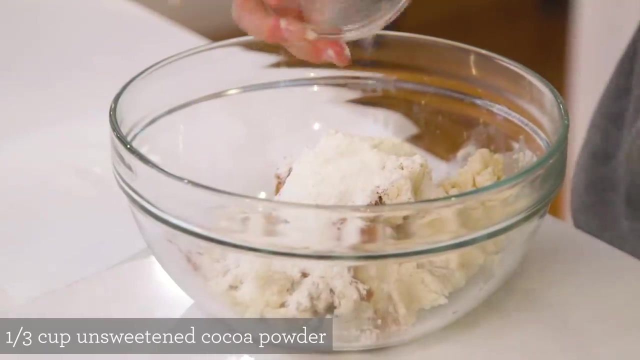 So you can start by putting your sugar cookie dough in a bowl. Then you can start adding some flour to it. You can start kind of mixing it around, And now I'm going to add some cocoa powder and the rest of my flour. It's really soft. I'm looking for white to try to mix it all in. 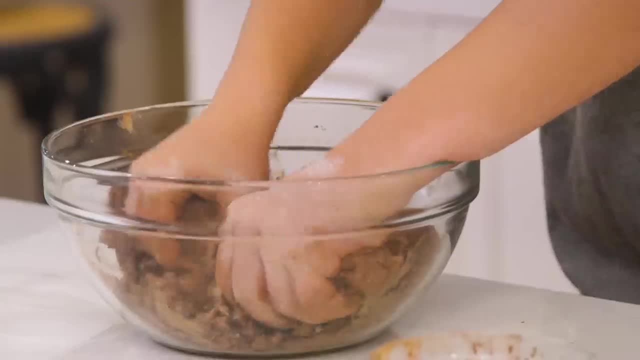 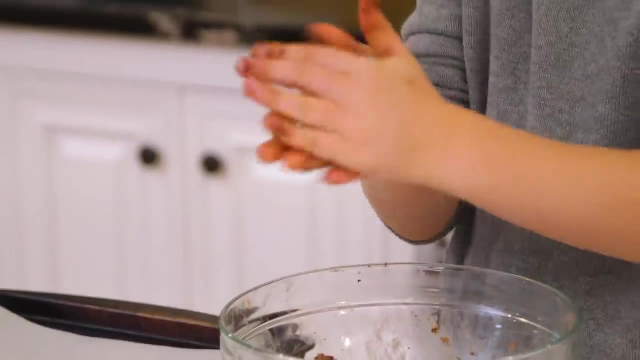 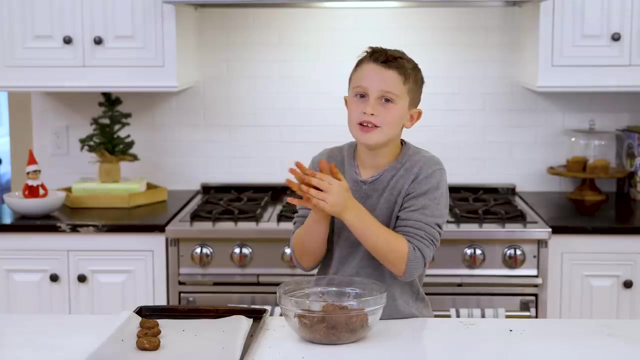 It takes some muscles, but I got plenty of those. Now we're going to take about a teaspoon of our dough. We're going to roll it up. It could be good to wash your hands right before you do this. Try to flatten them up a little bit. I'm just going to continue on until my baking sheet is full. 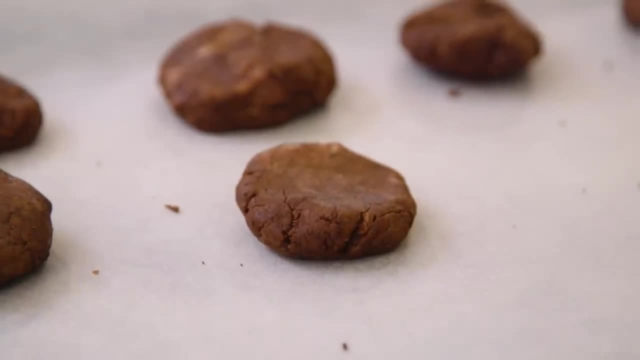 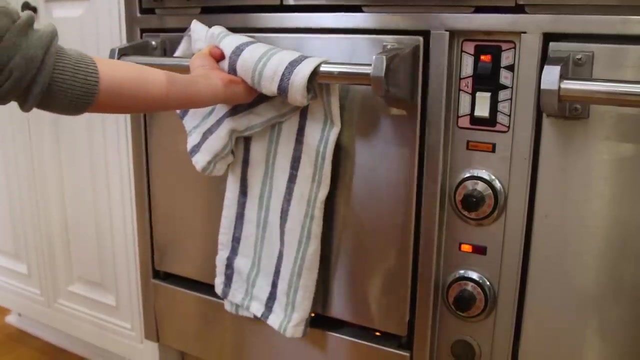 I just wish I could eat these right now. This one's perfect size, perfect shape. Now we're going to put this into a 350 degree oven for eight minutes. While our cookies are in the oven, we're going to cut some marshmallows in half, because you can't have hot cocoa. 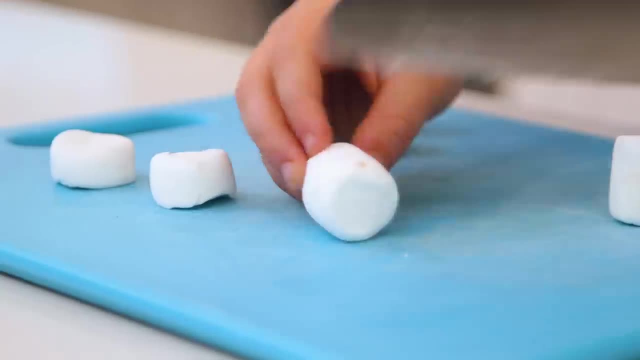 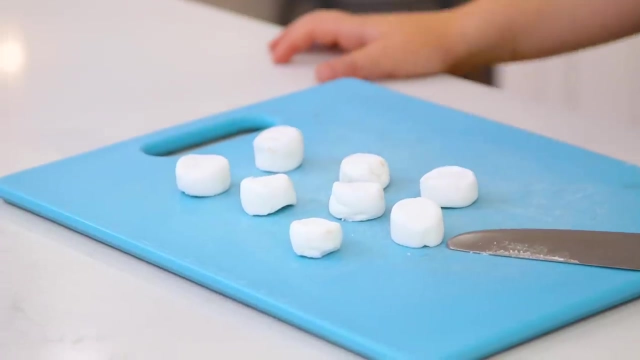 Without a marshmallow. I had eight cookies, and eight divided by two is four. It's easier to cut them in circles, because then you can put them on your cookies like that. All right, next we're going to melt some chocolate, So I've got chocolate chips. 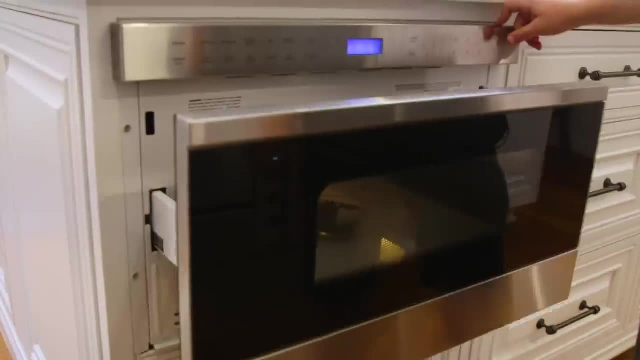 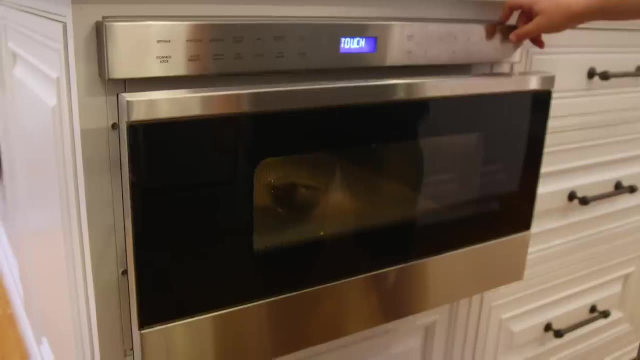 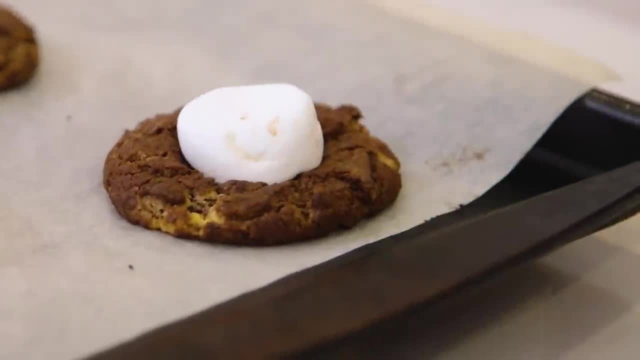 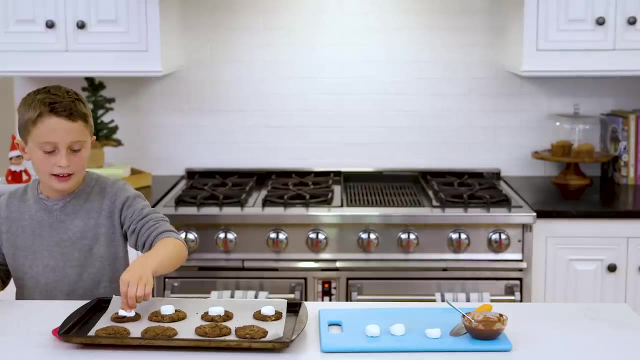 I'm going to take my half marshmallow and put it, place it on a cookie. They look so good. already That one looks good. I like the big ones that are like tall, because then the marshmallow kind of gets like stuck in it. Looks like I did some good math. 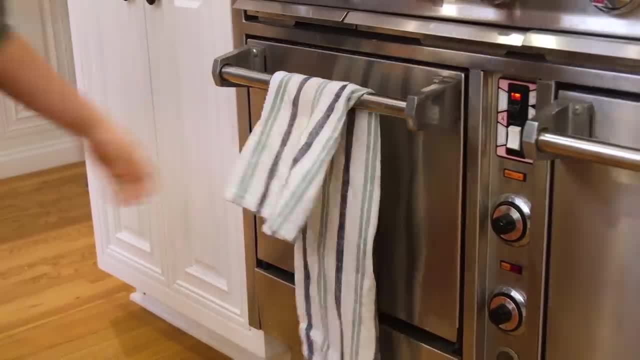 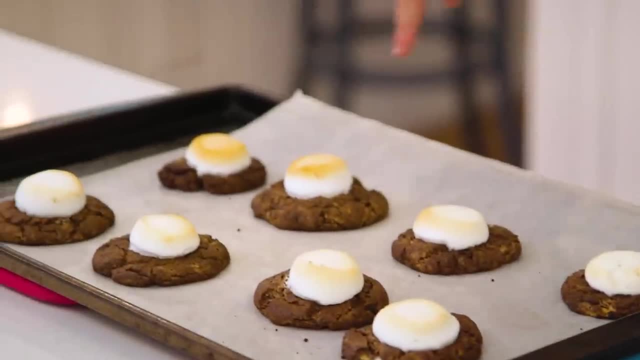 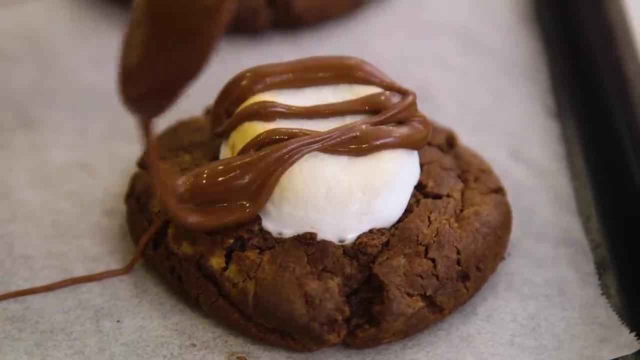 Put it back in the oven for two to three minutes till golden brown. All right, my hot cocoa cookies are out of the oven. They look so good, but I love those. This one, I think, is my favorite one that I made. Now I'm going to put some melted chocolate on a couple of them. I'm not going to cover the whole. 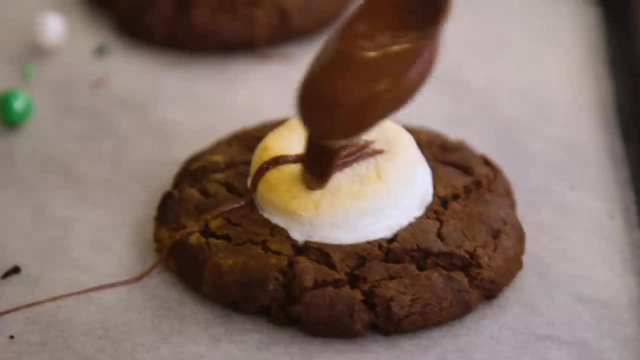 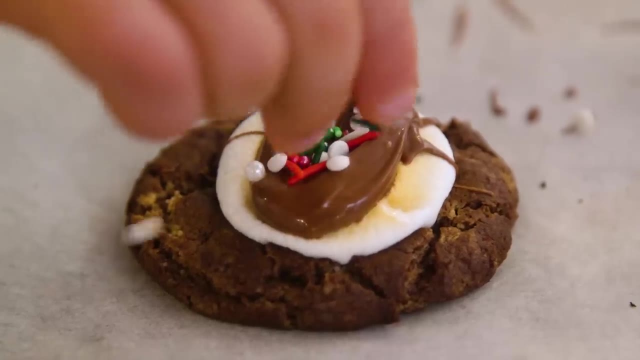 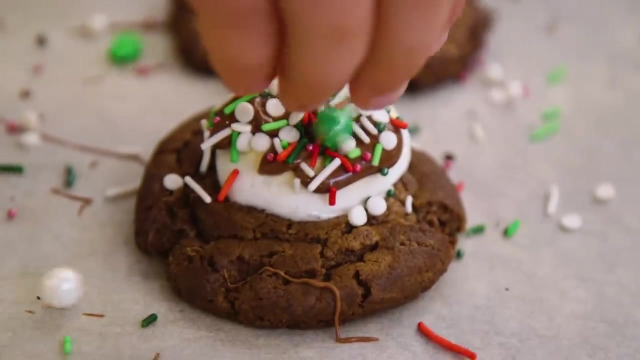 marshmallow. I think that's enough. I'm getting chocolate everywhere, but that's fine. Before my chocolate hardens, I'm going to decorate. So I got some leaf sprinkles. You can never have too many sprinkles, and that's a rule. I think I pretty much nailed this. These hot cocoa cookies are perfect on a cold winter day. 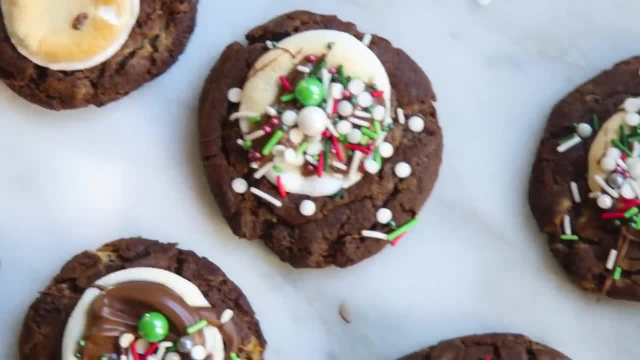 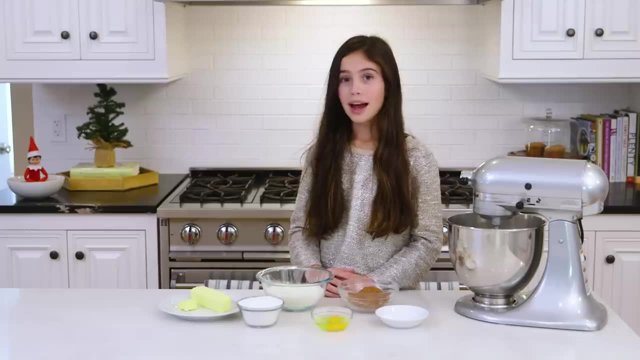 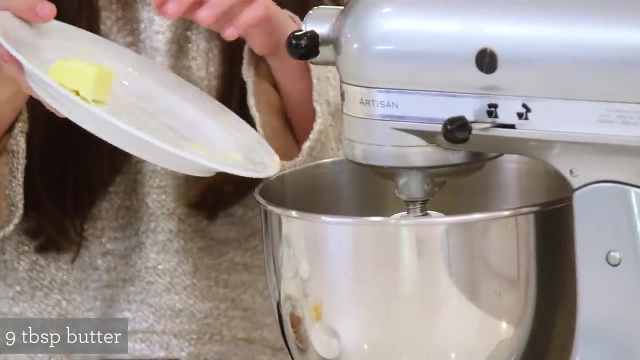 These hot cocoa cookies are perfect on a cold winter day, As delicious as they look. You'll have to trust me on that. Finally, we're making peppermint Oreos. I learned to make these at my cooking class. To get started, we're going to take softened butter. I'm going to put it into our mixer. 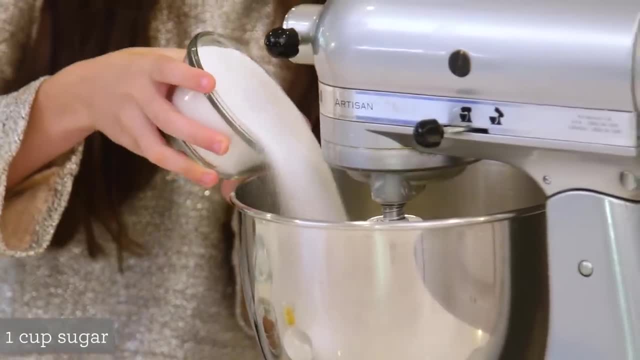 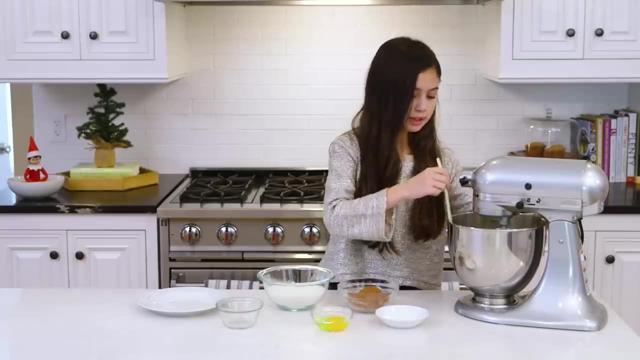 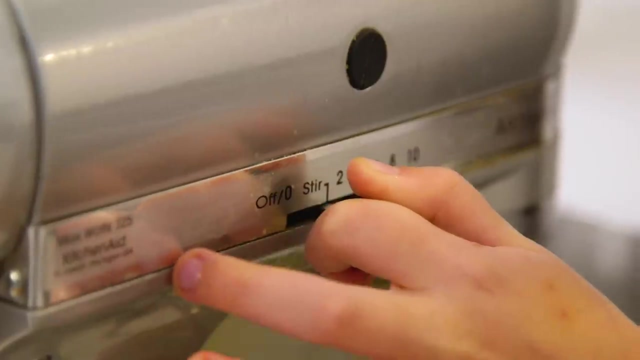 Don't worry, I washed my hands. Next, we're going to put our sugar in, and now I'm going to cream it. I'm just going to scrape down the sides so I can get everything in there. I'm just going to put in my egg. I'm going to turn it back on for just a few seconds. 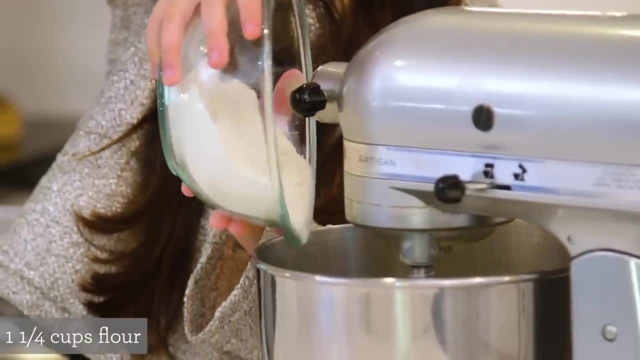 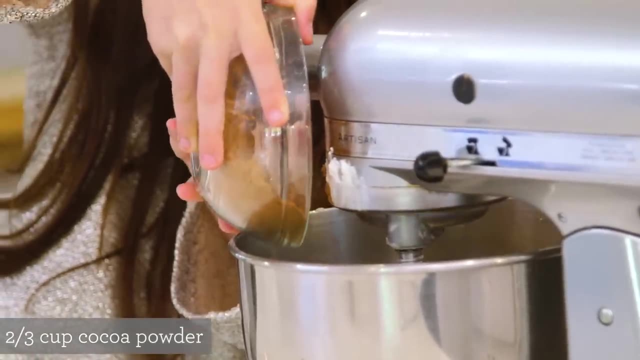 And now I'm going to put in my flour. I want to make sure that it's off. while you put in your flour, I'm going to put in my cocoa powder. So when you start stirring, you have to be careful, like to put it on slow, because it's going to splash. Now I'm going to put my baking soda. 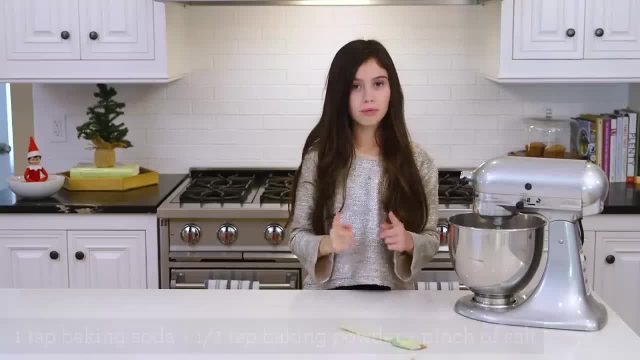 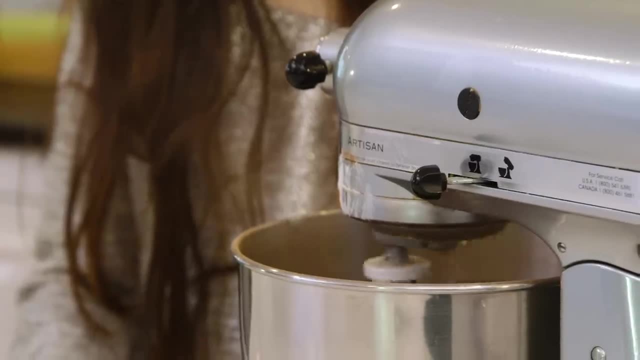 baking powder and salt. I'm going to stir it again. Remember we have to do it slowly or else it's going to splash. That's the cocoa powder. If you could see all this like, it smells good too. This is how it's supposed to look. 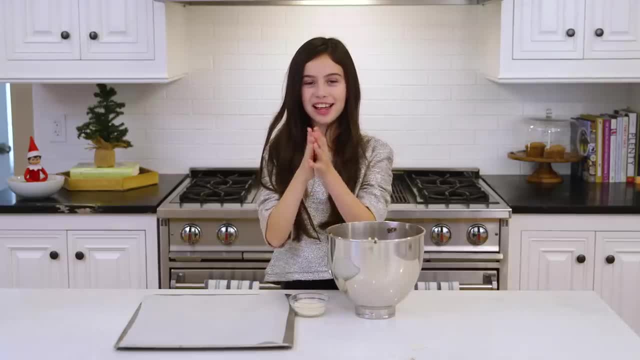 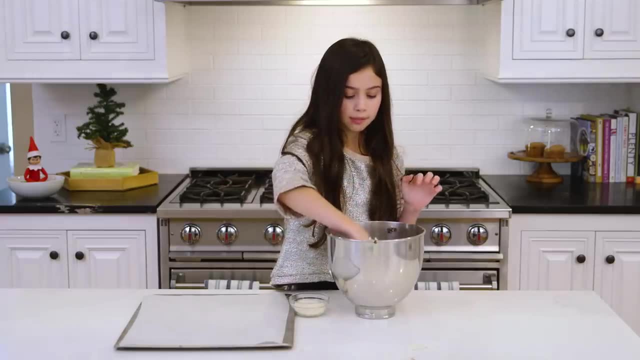 Now is the fun part. Let's roll back our sleeves and start getting messy. So you can either use an ice cream scoop or your hands, but I like to use my hands. So you take a bit of the dough and then you roll it into a ball, Then you roll it around. That's a lot. 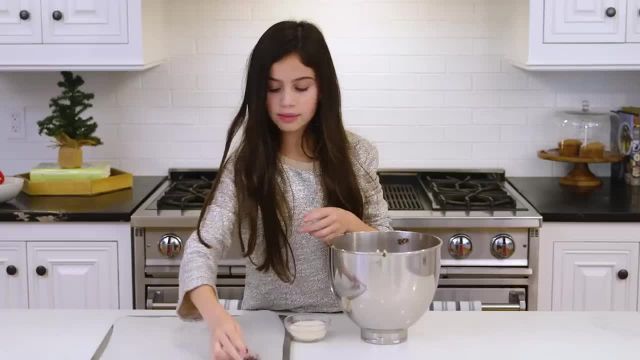 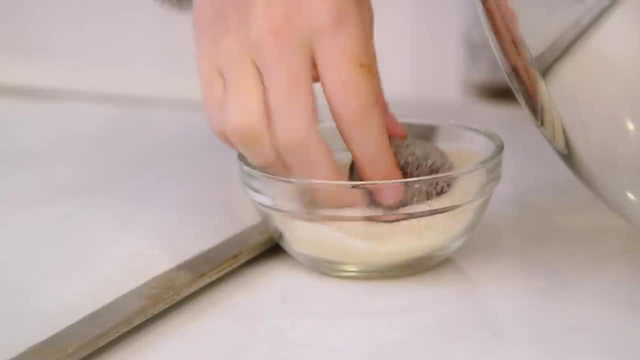 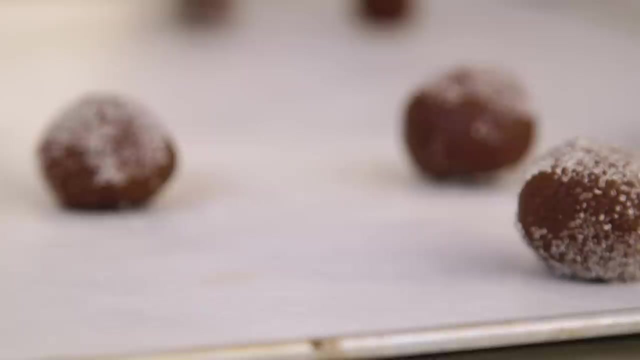 Then you put it on, but you want to leave spaces in between because these grow this big, That's really big. We just keep on doing this over and over again. You want to try to make at least two around the same size, because an Oreo has two halves. You don't want a lopsided Oreo. 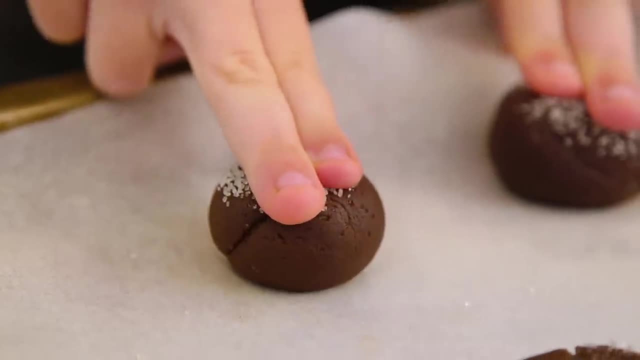 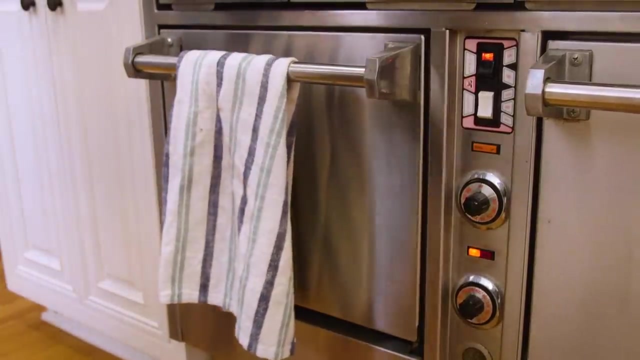 That looks like a snowball. Now I'm going to use two fingers to push them down. We're going to put them into a 375 degree oven for six to eight minutes. While our Oreos are cooling, we're going to make the filling. 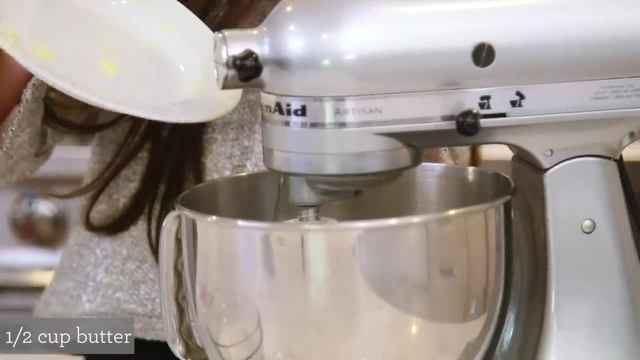 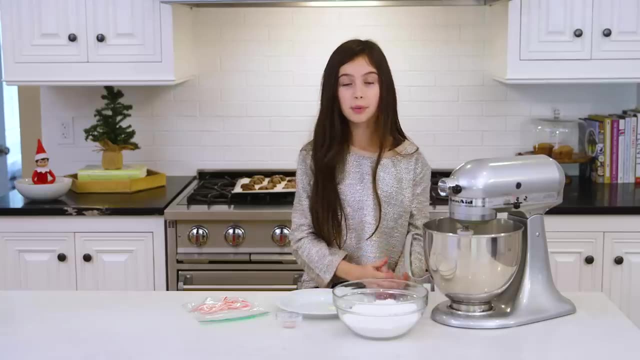 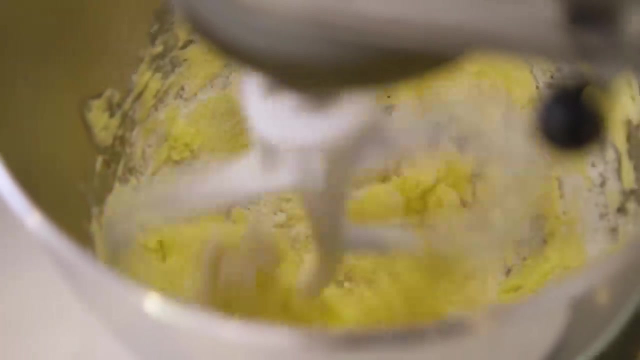 And we're going to start by putting some softened butter into the mixer. It's pretty whipped, and now we're going to add powdered sugar a little at a time, And now, with it running, we're just going to add a little bit more. 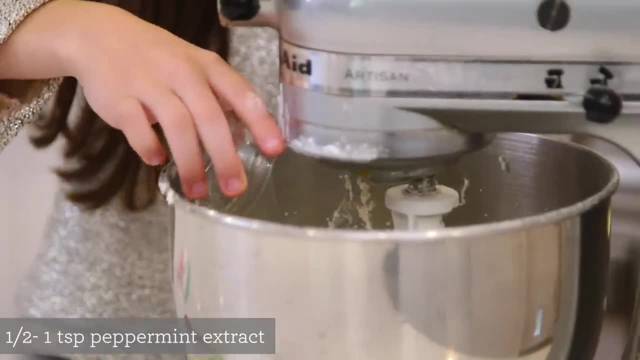 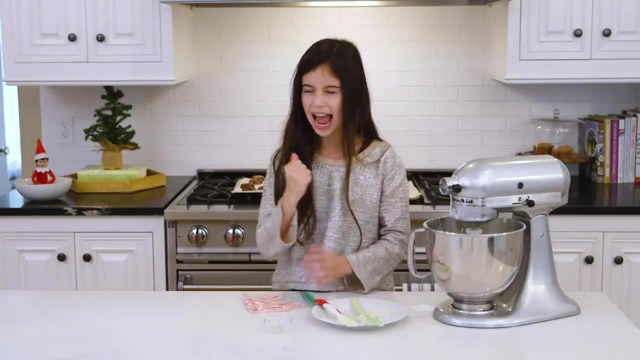 I'm just going to add a little bit of powdered sugar, Peppermint extract, And then I'm going to add in these candy canes that I'm about to crush. Little tip: don't do it with your hands. There we go.